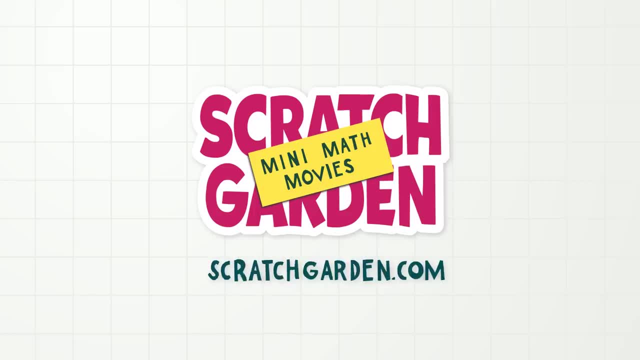 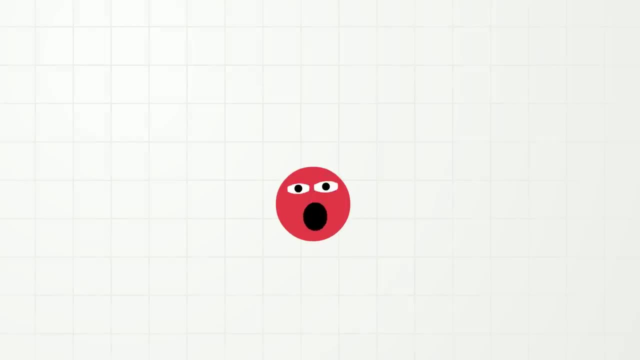 Oh, hi everybody. Today I'm going to talk to you about numbers and fractions and maybe even Kevin. Huh, I really like Kevin. Okay, so we all know how to count things right? Yes, of course you do, But do you know how to count parts of things? I will show you. 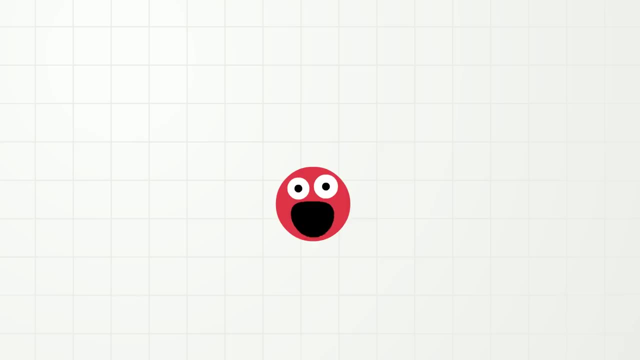 First, we need something that we can count and also divide into equal parts. Uh, how about a pizza? Oh, no, not another pizza example. Hmm, we need something else. How about me? Oh, good idea. Okay, so now, how many me's do you see? That's right, there are one, two. 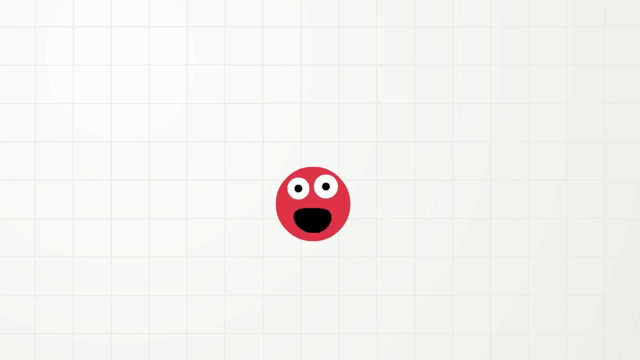 three me's. And now, how many me's do you see? Yes, there is just one me, One whole me. Yay, But now watch closely. but don't worry, I am a cartoon, so it won't hurt. How many me's do you see? 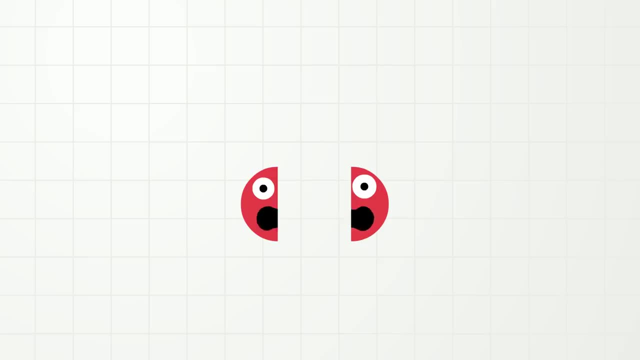 Are there two me's? No, not really. There are two parts of me or two equal halves of me, One half here and one half here, And when we put one half and one half together there is one whole me. So in math, when we have parts of whole things like this, we can call: 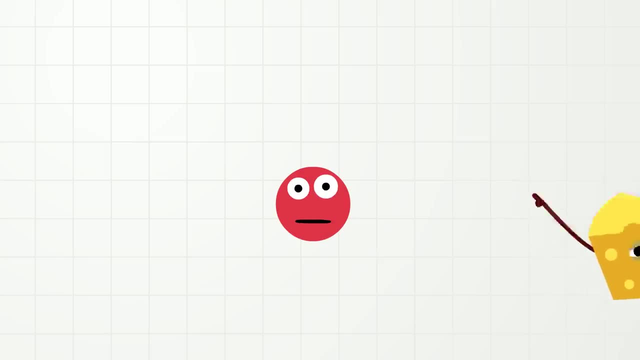 these parts: fractions, Fractions. Okay, you did such a good job listening. it is now time to sing a song. Okay, that's enough. So, as I just showed you, if I divide myself into two equal parts, then I have two halves. But what happens if these halves also get? 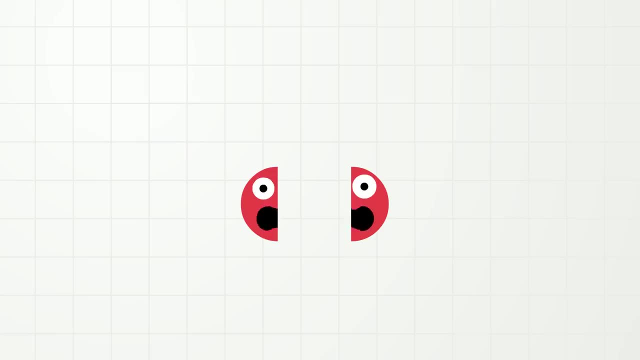 divided into halves. Okay, watch, And don't worry, I am a cartoon, so it won't hurt. So now are there four of me? No, not really, but there are four equal parts of me, So we can call them fourths. 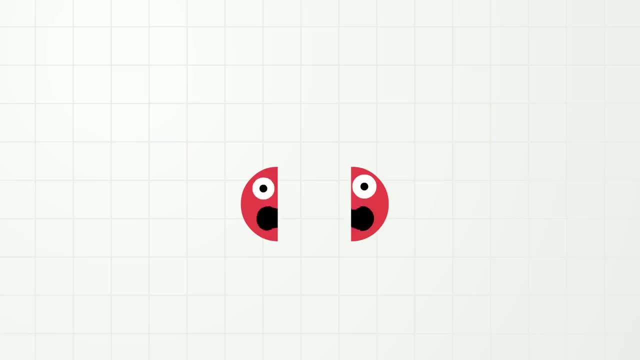 divided into halves. Okay, watch and don't worry, I am a cartoon, so it won't hurt. So now are there four of me? No, not really, but there are four equal parts of me, So we can call them fourths Forth. 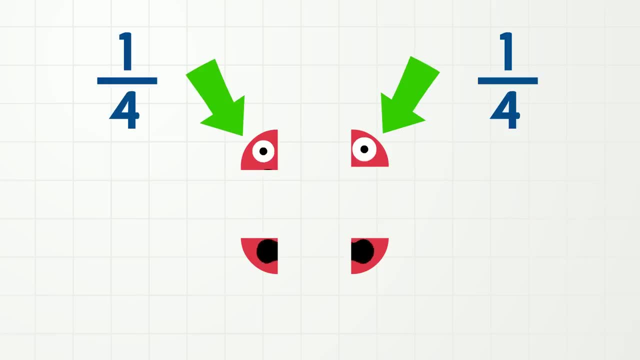 One fourth here, One fourth there, Andro, One-fourth here, one-fourth here and one-fourth here. We can also call a fourth a different word, and that word is quarter Quarter, So one-quarter here, one-quarter here, one-quarter here and one-quarter here. 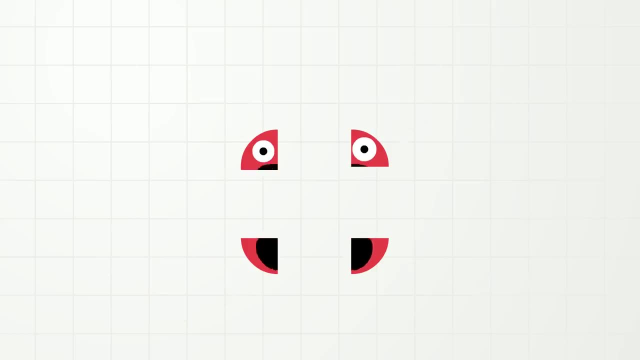 And if we put four-quarters or four-fourths of me together, there is one whole me. Okay, let's review, because it might be a little confusing. Uh-oh, where did I go? Don't worry. So this is one-fourth of me, or one-quarter. 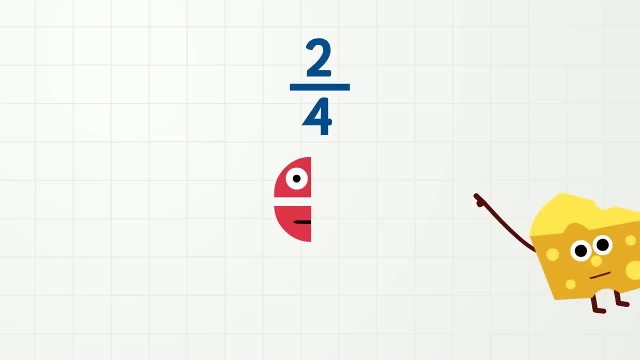 This is two-fourths of me or two-quarters, And two-fourths is also the same as one-half, One-half. This is three-fourths of me or three-quarters, And this is four-fourths of me or four-quarters. 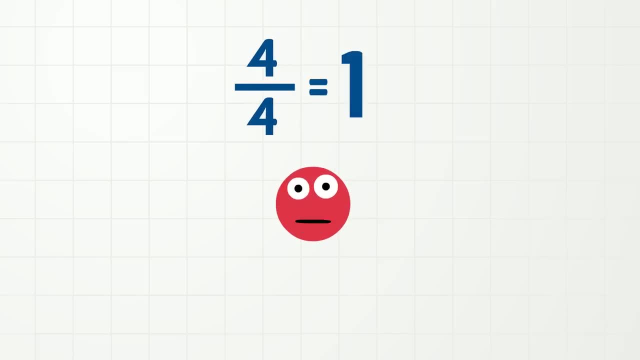 And four-fourths is the same as one-whole, One-whole. Phew. you did such a good job listening. it is now time to sing a song. Okay, that's enough. Let's talk about something else besides me. 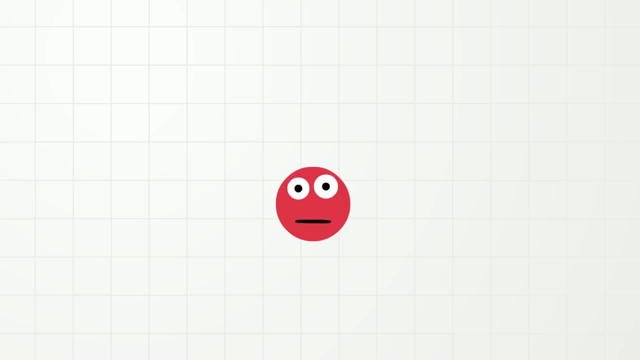 Do you know when is another good time to use fractions? When we are sharing something, Especially if we want to share something fairly and give everybody the same amount. Let's use something to help us explain What can we use, Hmm. 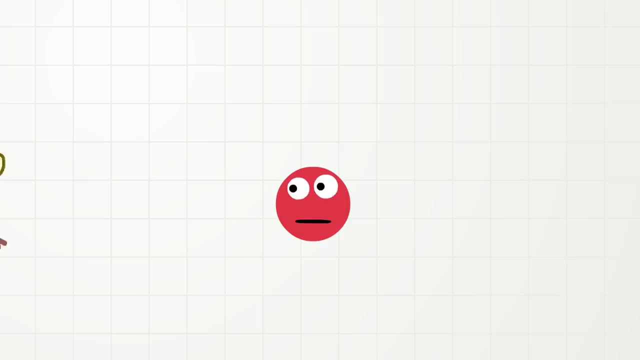 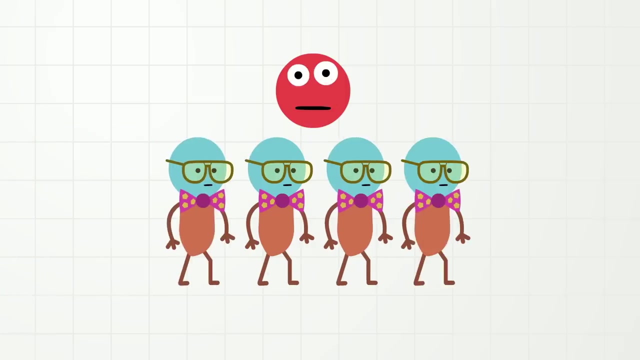 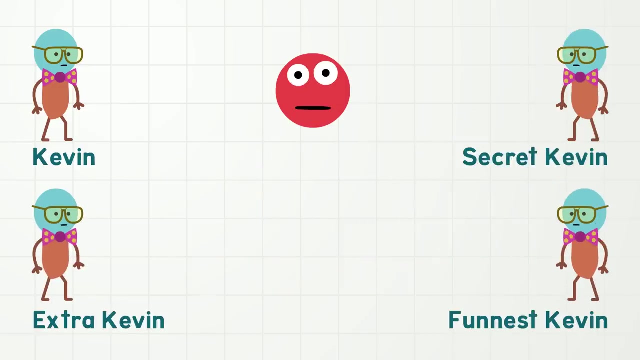 Oh, I know How about Kevin. It's a Kevin. No, I want all the Kevins. Okay, here we have four Kevins: Kevin, Extra Kevin, Secret Kevin and Funnest Kevin. What if we have eight cookies and we want to share these cookies fairly to all the Kevins? 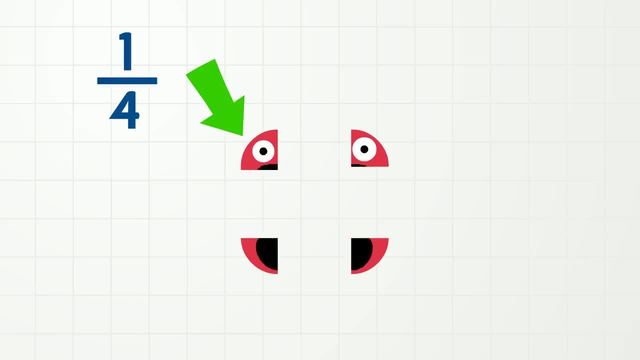 Forth, Forth, Forth, fourth here, one fourth here and one fourth here. We can also call a fourth a different word, and that word is quarter, quarter. So one quarter here, one quarter here, one quarter here and one quarter here. 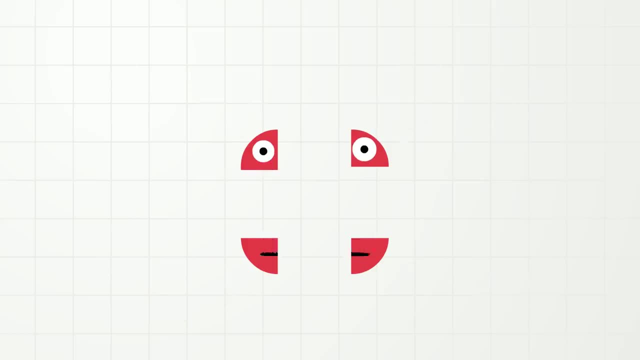 And if we put four quarters or four fourths of me together, there is one whole me. Okay, let's review, because it might be a little confusing. Uh oh, where did I go? Don't worry. So this is one fourth of me, or one quarter. 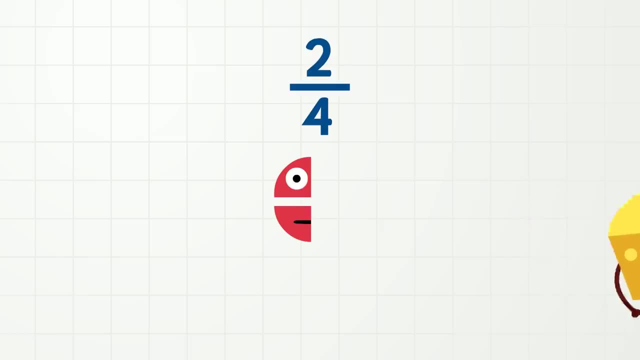 This is two fourths of me, or two quarters, And two fourths is also the same as one half, one half. This is three fourths of me, or three quarters. Okay, And this is four fourths of me, or four quarters. 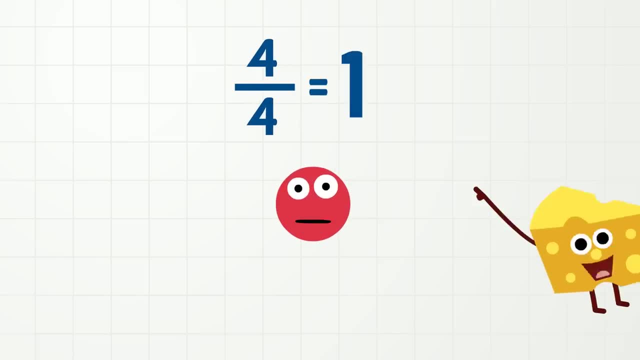 And four. fourths is the same as one whole, one whole. Phew. you did such a good job listening. it is now time to sing a song. Okay, that's enough. Let's talk about something else besides me. Do you know when is another good time to use fractions? 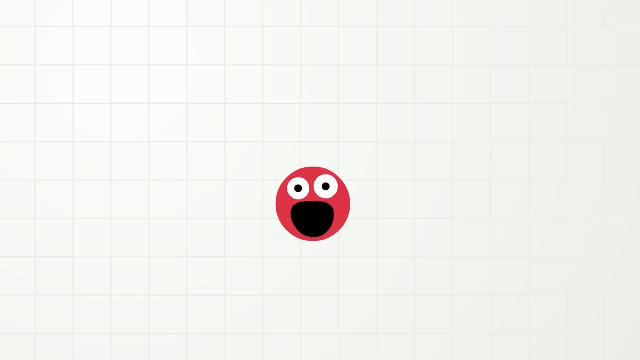 When we are sharing something, Especially If we want to share something fairly and give everybody the same amount, Let's use something to help us explain. What can we use, Hmm, Oh, I know How. about Kevin? It's a Kevin. 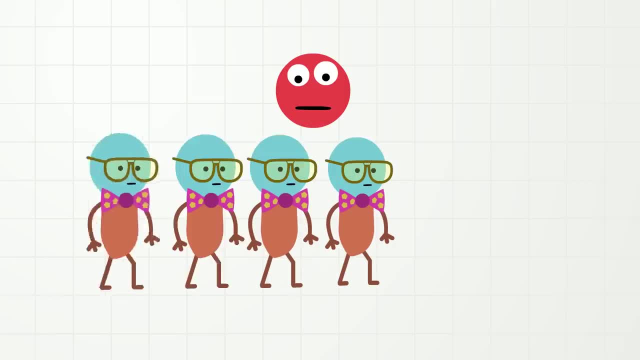 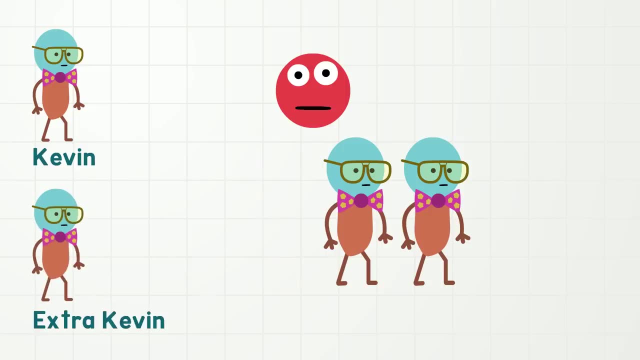 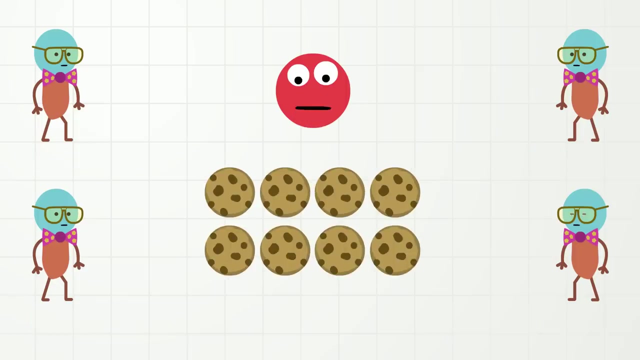 No, I want all the Kevins. Okay, here we have four Kevins: Kevin Extra Kevin, Secret Kevin and Funnest Kevin. What if we have eight cookies and we want to share these cookies fairly to all the? 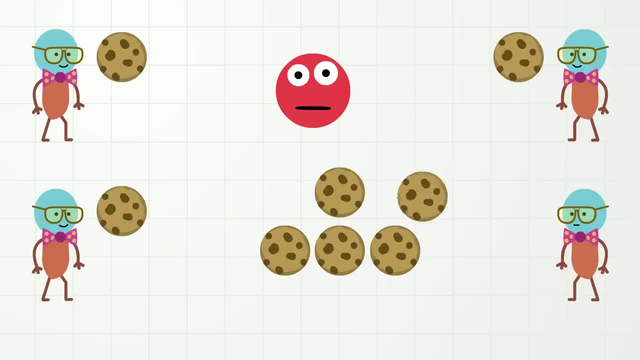 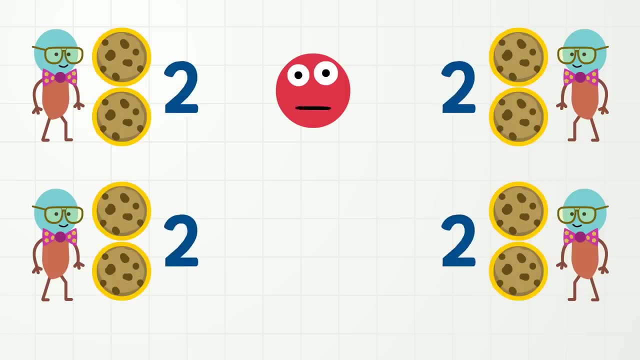 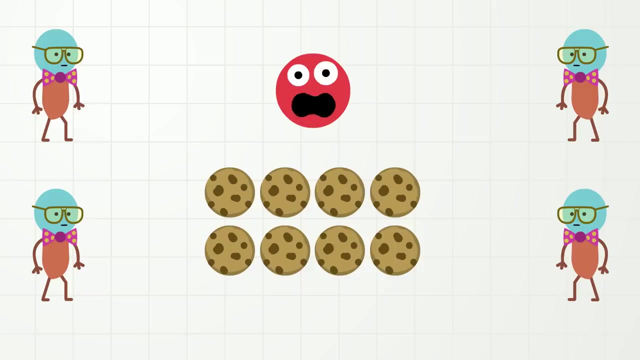 Kevins, Let's try Move cookies. Okay, now each Kevin has the same number. One, two cookies. Come back cookies. Now what happens if two of these cookies disappear? Dennie whimpers, Yep. 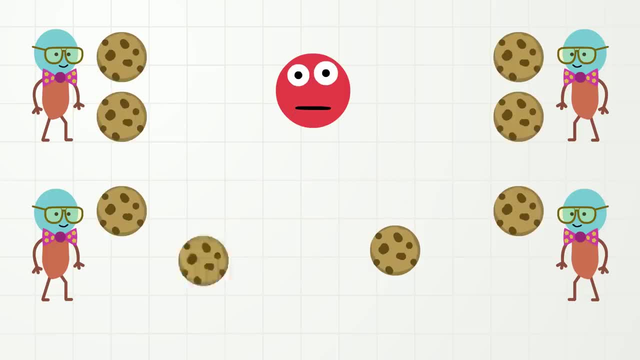 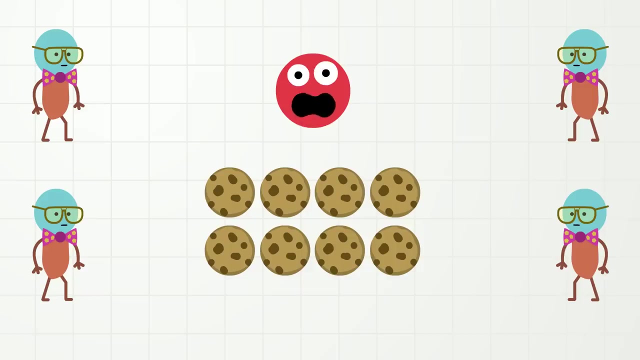 Let's try Move cookies. Okay, now each Kevin has the same number: One, two cookies. Come back cookies. Now what happens if two of these cookies disappear? Caw-caw-caw-caw-caw-caw-caw-caw. 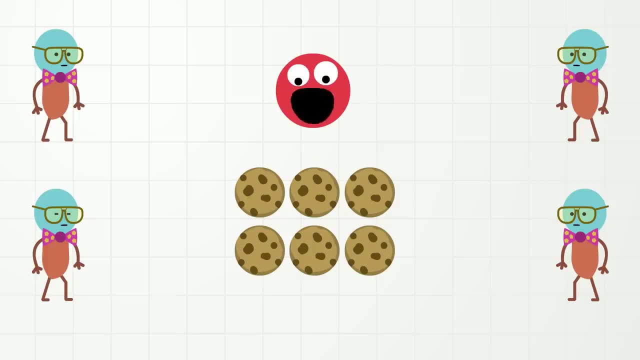 Caw-caw-caw-caw-caw-caw-caw-caw-caw-caw-caw. Well, that means we only have six cookies left. Let's try and share them Now. each Kevin has one cookie, but there are two cookies left. 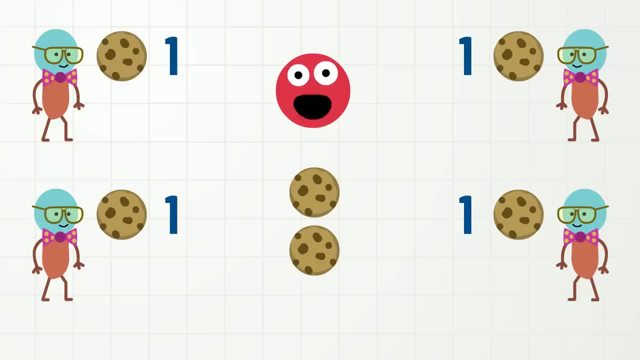 How can we share them fairly? It looks like we're going to have to make some fractions and break the cookies in half. Now each Kevin has one cookie and one half of a cookie. Caw-caw-caw-caw-caw-caw-caw-caw-caw. 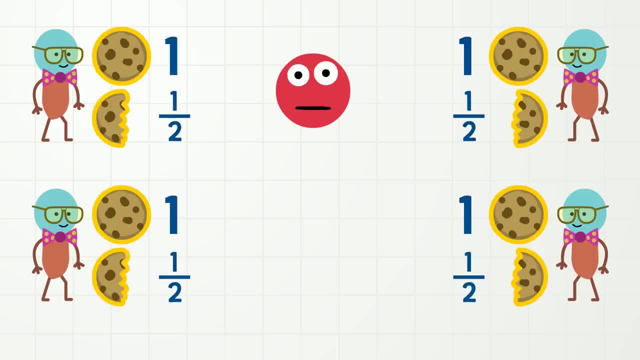 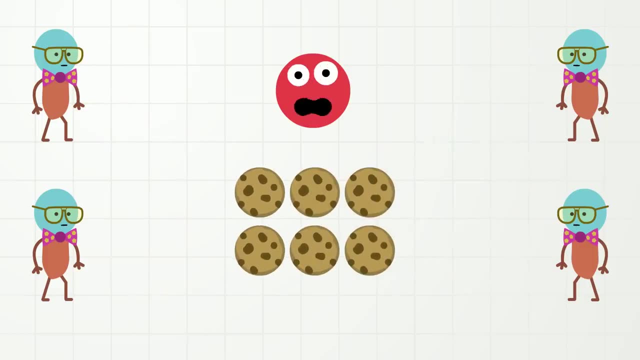 One and one half cookies each. Okay, come back cookies. Okay, now what happens if five more of the cookies disappear? Caw-caw-caw-caw-caw-caw, Caw-caw-caw-caw-caw-caw-caw-caw-caw-caw. 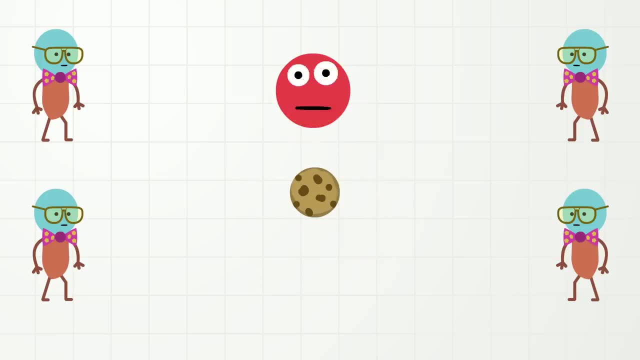 Caw-caw-caw-caw-caw-caw-caw-caw-caw-ca. That means we only have one cookie left. Let's try and share them…. Hey, how can we share one cookie fairly? Caw-caw-caw-caw-caw-caw-caw-caw-caw-caw-caw. 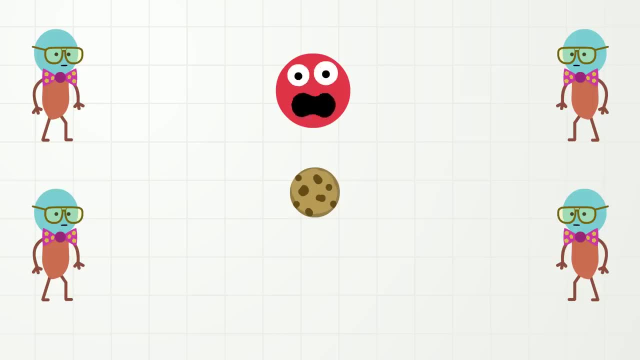 One and one half cookies each. It looks like we are going to have to make some fractions and break the cookie into quarters. Now each Kevin has one fourth or one quarter of a cookie. Don't be sad, Kevins, you got one quarter of a cookie. 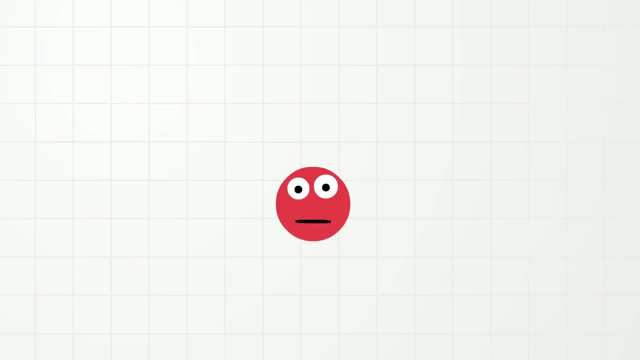 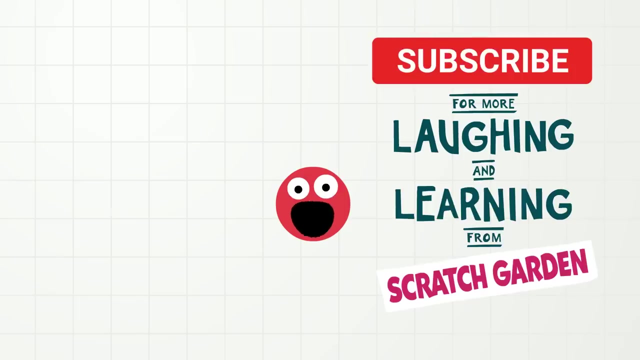 OK, that is all the time today we have for fractions. Don't forget to subscribe to our channel for more laughing and learning from Scratch Garden. Did you know that we have another video where we split words into parts? Yeah, we do. It's called syllables.